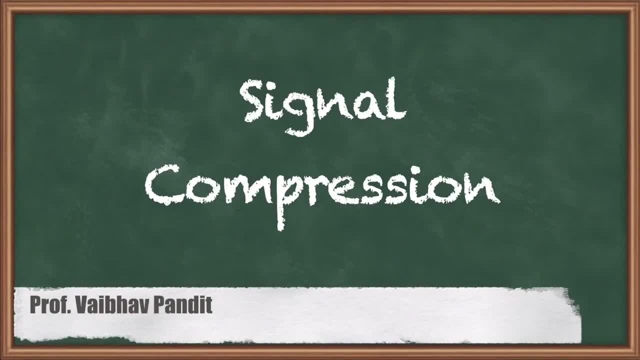 Hello friends, and welcome to this video. We are with the last chapter of advanced digital signal processing. The chapter title is applications of signal processing. So the various popular applications those are possible because of the potential working of signal processing methodologies, those we have learned in the previous chapters we are having a discussion on This, can be listed as signal detection, then spectral analysis, which we have seen for the three types of signals. 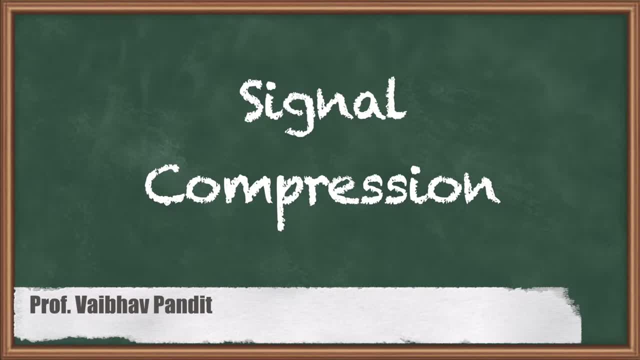 Signs: sinusoidal signals, speech signals, random signals. Next to that, we have also seen musical sound processing, along with how the music synthesis can be there in digital way. In the previous video we have seen the analytic signal generation And now let us have a discussion on very popular and important application of signal processing domain that it is compression, As we know that we can have compression of the signal. 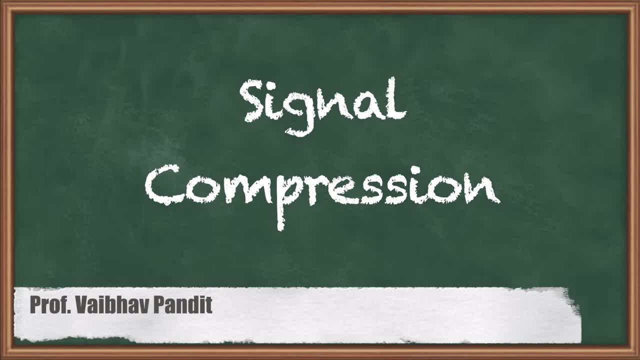 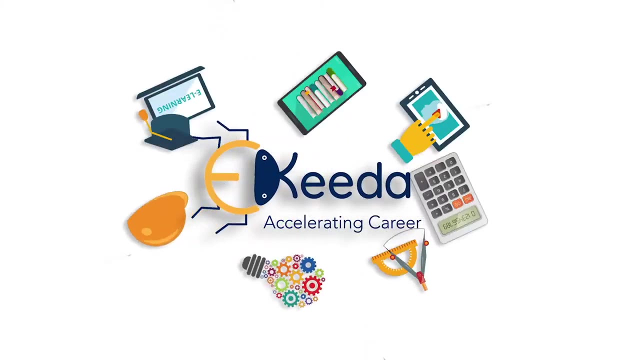 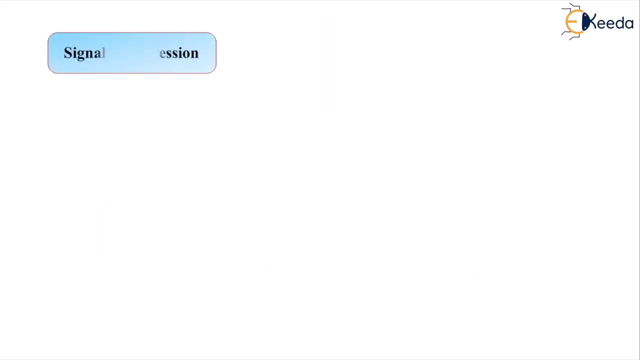 Having the benefit of saving the memory storage and also saving the bandwidth while having that transmitted from one place to another. So let us discuss with respect to signal compression. So let us begin with the topic. So here we start with our topic. the topic titled signal compression. 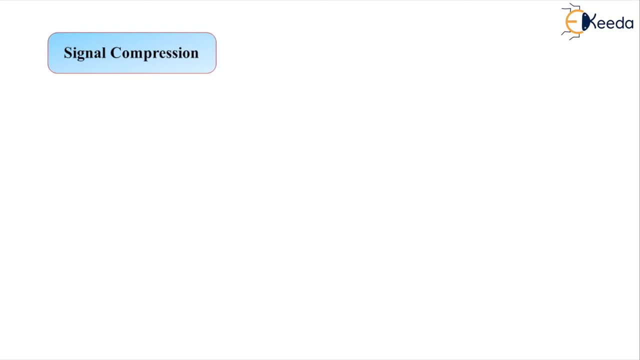 So, as our subject is advanced digital signal processing, So one must know that what exactly the signal mean. So the simple short answer can be: signals carry information. So whatever the kind of information is there, in a variety of forms it may be, You can call it to be a signal and that you should be able to have represented with the mathematical tools we have learned so far. 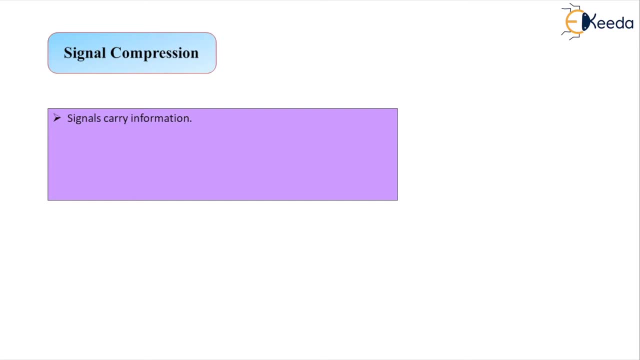 And then, whatever the methodologies of digital signal processing are We have learned, we can make them applied to that information, What we have called a signal, and then we can achieve our application with good efficiency. So what is the objective of applying digital signal processing techniques? 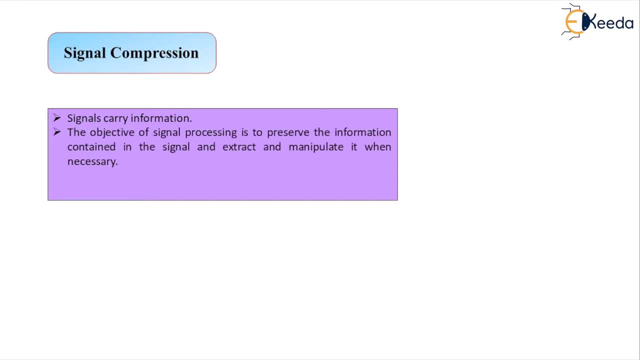 That to preserve the information contained into the signal and also to extract and manipulate it whenever it is necessary. So let us say, If we take the example of two dimensional signal that we call to be image, here So we have different kinds of images. 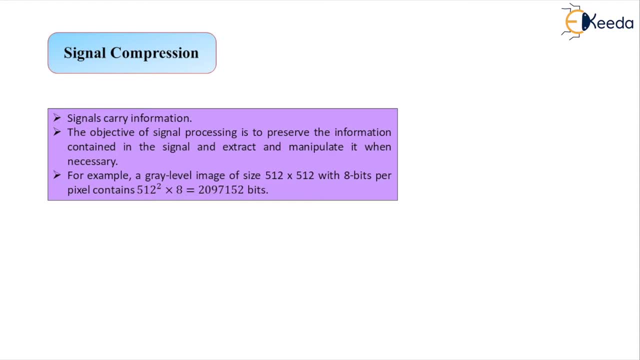 We can have binary image when the representation of signal information is in terms of zero and one only. We can have grayscale image. We can have color image. So, for example, if we talk about the grayscale image, So as it is a two dimensional signal, 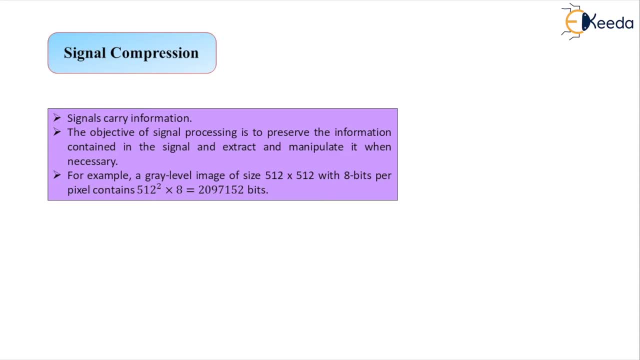 So we can have the representation, The representation of image into number of rows and number of columns And, specific to a certain row and certain column, We come to a location, what we known to as a pixel, into that image. So let us have the total size of 512 pixels by 512 pixels. 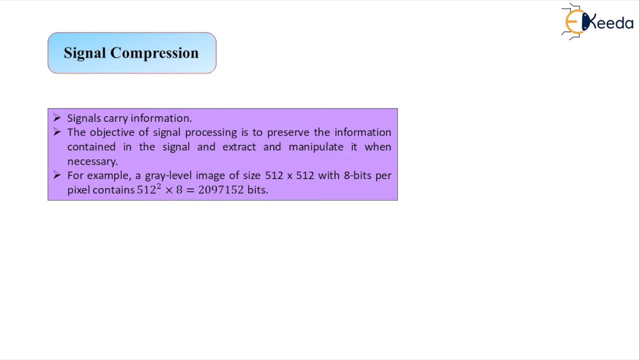 And the representation, as it is gray level type of the image, is with the help of n bit. Here, in this example, We are considering 8 bit representation Per pixel, So this is containing 512 multiplied to the same dimension on other side. 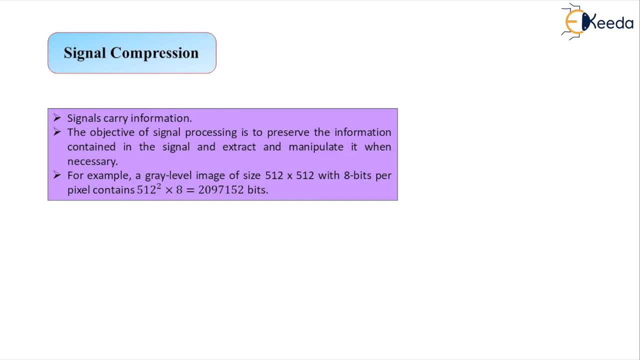 That is why we represent square of 512 multiplied to 8 bits per every pixel. So this multiplication is resulting into the figure: We have 2097152 bits here. So let us have the grayscale image visualization. So let us see: This is a flower in the grayscale visualization. 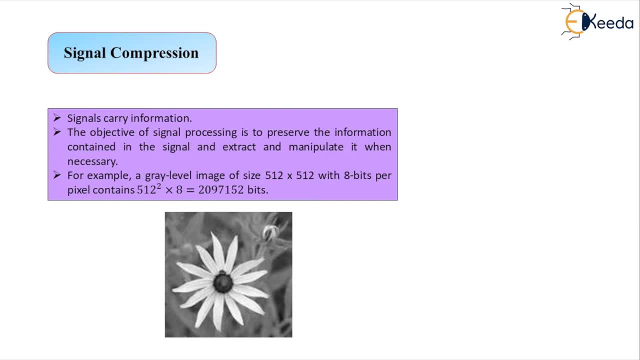 As you see the image plane to be of square type. It means the number of rows is equal to number of columns. Here we have 512 by 512.. And for every pixel location there are requirement of 8 bits. So this is what the case. 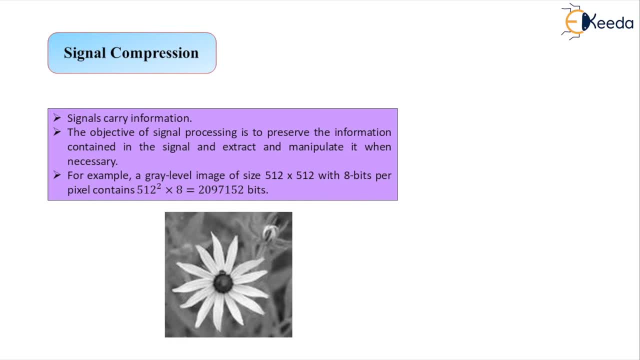 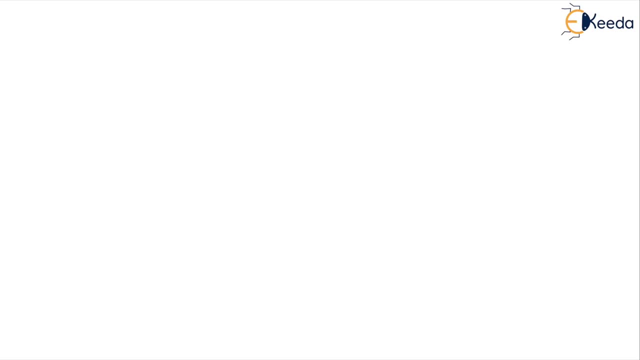 Now if we want to convey the information that we have picturized into the grayscale form Instead into the color form. So what can be the scenario? A color image for the same scenario for the same dimensions? If we are representing, We know that the color image will be a stack of three such image planes corresponding to red. 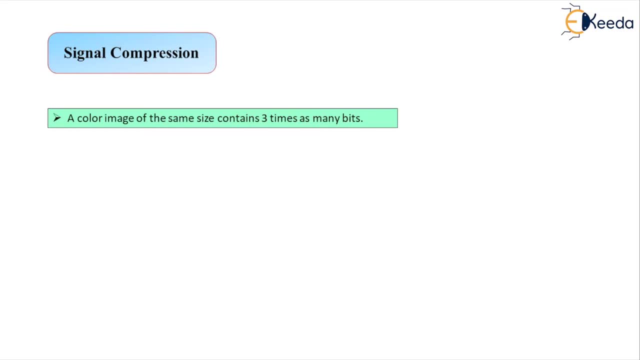 Green and blue frequency bands here, So that it will be RGB color image. So now the requirement of how many bits we need for representation, for storage and further communication of this particular image signal from transmitter to the receiver will be three times greater than that of the earlier representation here. 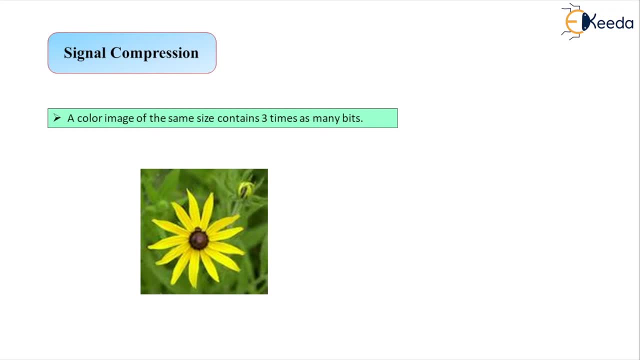 Now, here you see, the colorful representation of the same scenario, with the same dimensions, 512 by 512 pixels, And for every pixel we require 8 bits to represent, And there it will be the individual band of red, Then green and then blue. 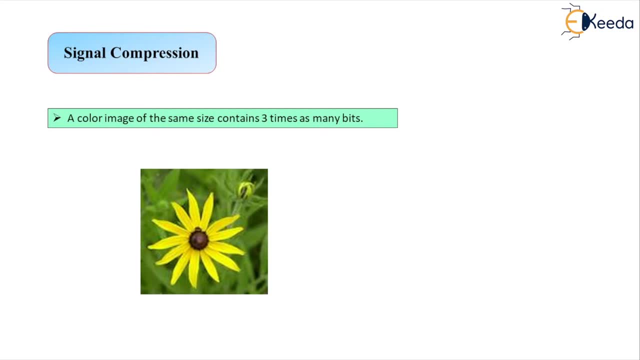 When they are stacked together. we get this pictorial representation here. Now what is the next thing? The next thing is that We require good efficiency for storage of the digital signals of this particular kind, And it is often necessary to have Compression of the digital signal. 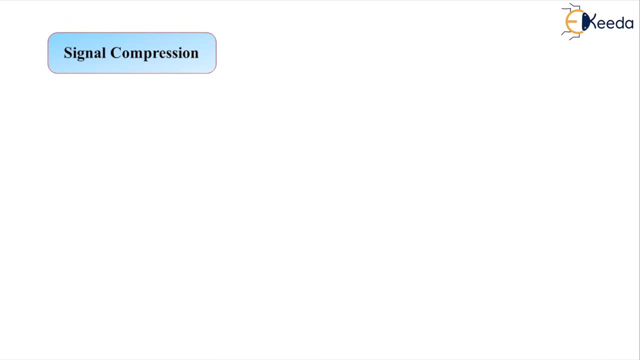 Compression of the data for saving the memory. And this compression of data is into the smaller size that requires significantly fewer number of bits. here. A signal into the compressed form also requires less bandwidth for transmission, as I have already discussed with you. So in short, signal compression is nothing but the reduction of the amount of the data. 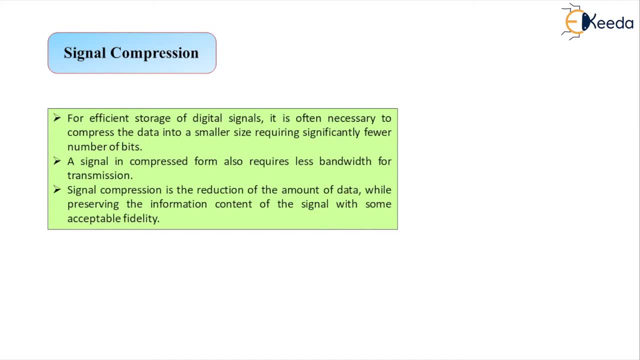 Along with preserving the information content of the signal With some acceptable fidelity. So here we are talking about fidelity. So whenever we have stored this information with minimal number of bits And we want to reconstruct back the original representation for any application at hand, 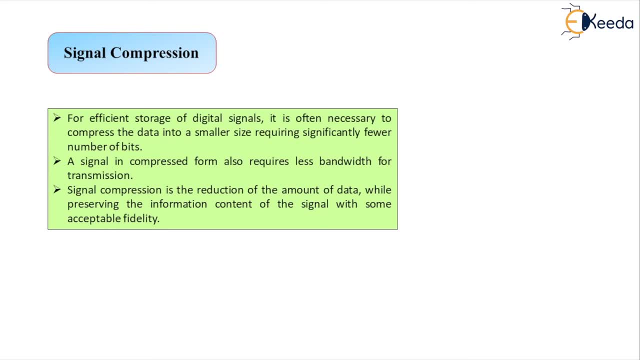 We should be able to do it with the coded form or the stored form of that information here Now, practically how it is possible- See The possibility of signal compression- is because Most of the signals are having a certain kind of data redundancy. So what is data redundancy? 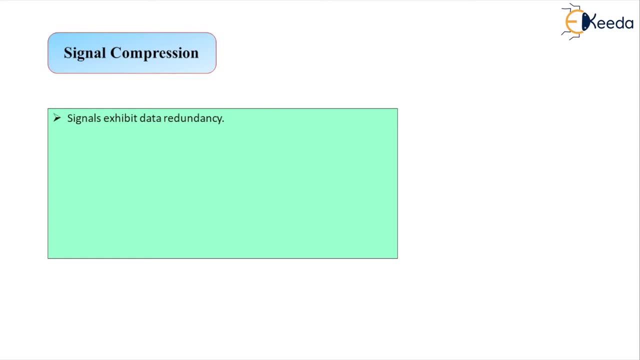 There is a certain kind of or certain amount of data That has no relevant information We are intended for, So such type of data can be removed here, So we can say that We can have reduction into the data redundancy And whatever the important things are. 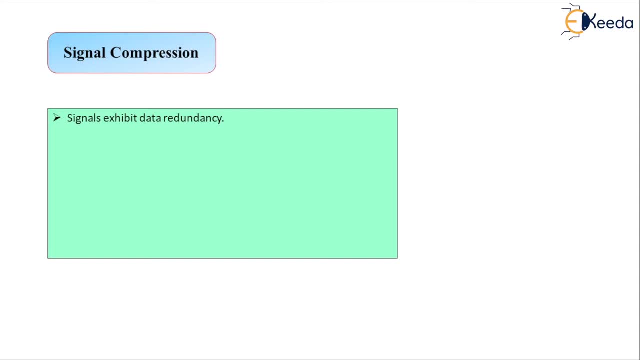 Only if they are taken into account We can have the signal compression possible. So there are basically three types of data redundancies Usually encountered into the practice. Those are coding redundancy, Then inter-sample redundancy And then the psycho-visual redundancy here. 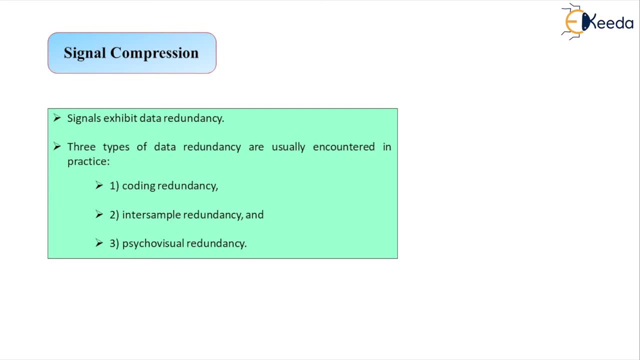 Now, at this point we are not going in much detail Because of how these are the variety of the redundancies, How the coding redundancy is different than the inter-sample And that of the psycho-visual redundancy. Now, in this video, I will just give you the brief introduction. 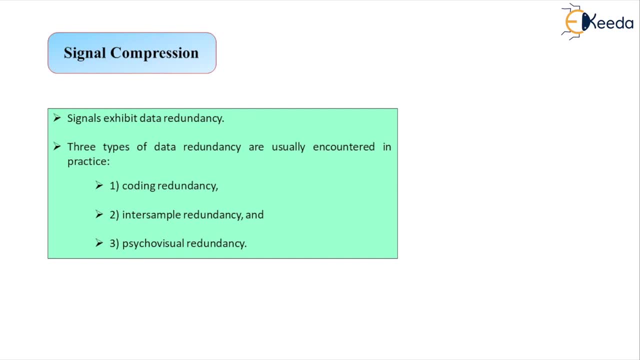 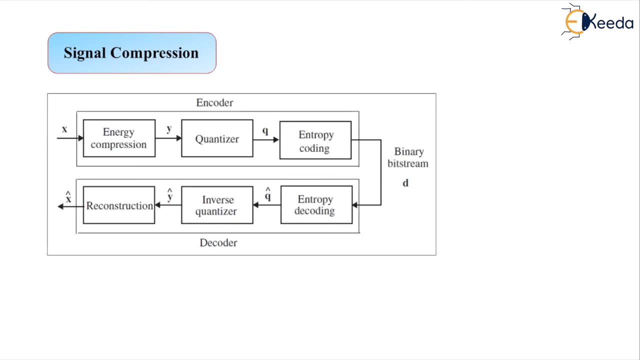 How the signal compression can be done. So for that purpose, Let us have the discussion with respect to a block schematic. So here we have the block schematic. So from this block schematic It must be clear to you people that The signal compression methodology 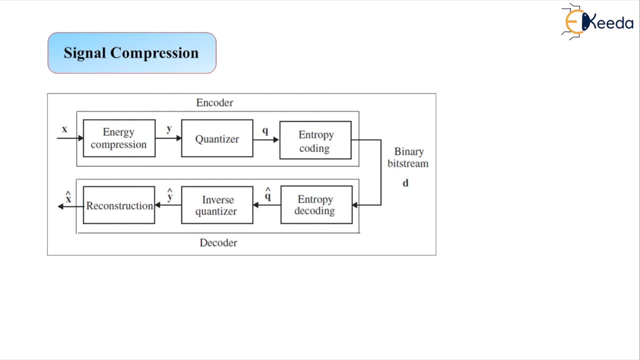 Can be separated into two major parts. One is for encoding purpose, Another is for decoding purpose. If you start with the original information to be compressed, The signal to be compressed, That it is represented as x, That is fed as input to the encoded part. 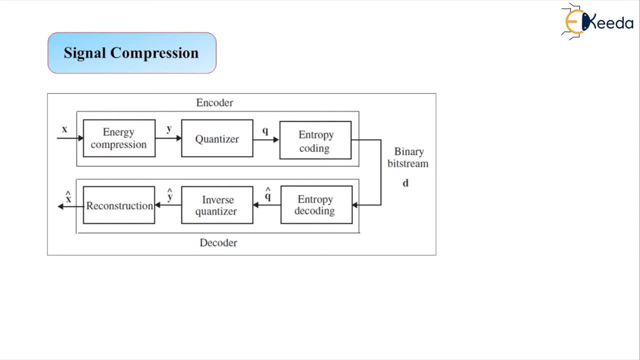 Where we have the sub-blocks as represented, Energy compression. So that will get x into the modified form As represented by y. Y is fed as input to further the quantizer. That will give you the signal representation at intermediate stage By small q here. 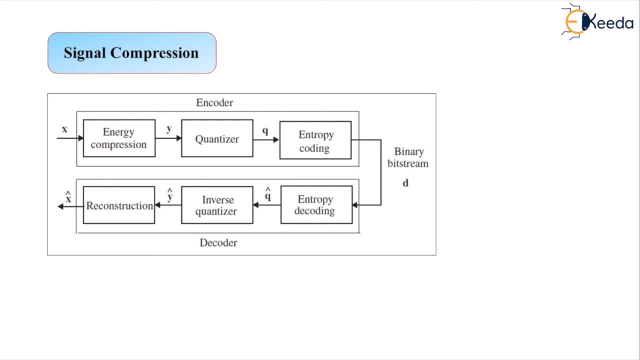 And then the entropy coding is performed To result into the representation of D, Which is the binary bit stream, And that it is the coded form here. So I can say that The signal x is compressed And D is the compressed form. 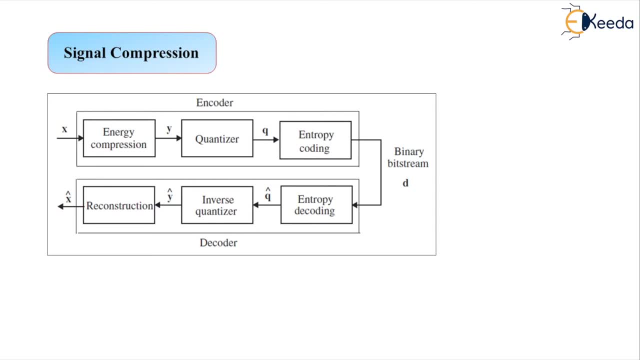 This is the representation of the original information here. So this way we have achieved the signal compression And whenever there, it is a requirement of Regenerating the original information From the coded form. So there should be good fidelity here, Good efficiency. in short, you can say: 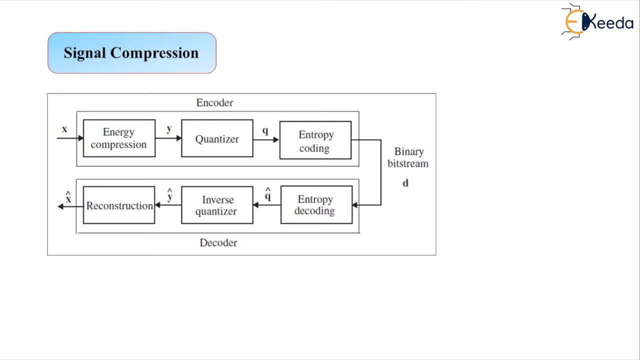 So there it is a reverse procedure To the encoding that we have Decoding in the below part here. So first of all the bit stream In binary form that is coded one Is fed as input to entropy decoding. That is resulting into the signal. 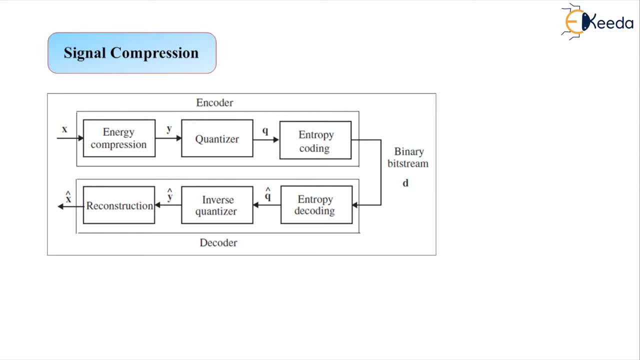 As denoted by q cap here. Then there it is inverse quantization, Which results into y cap, And finally the reconstruction of the information. So practically Most of the time it does not 100% match with the original information, But it is most of the time. 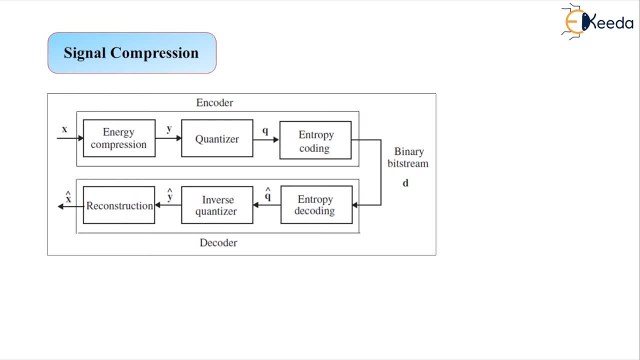 Similar to most percentage. That is why here we represent It with the help of x cap here. So in concern to the block schematic representation For the signal compression And decompression Methodology I see here, Let us discuss few of the important formulae. 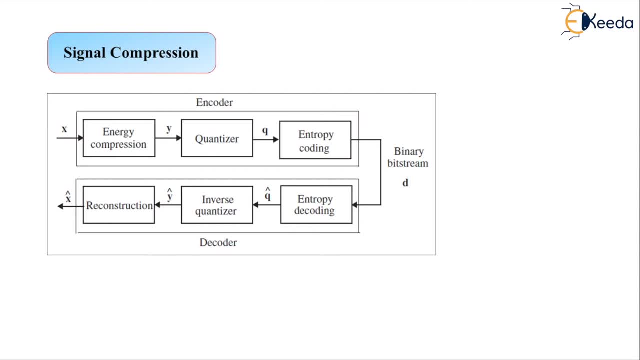 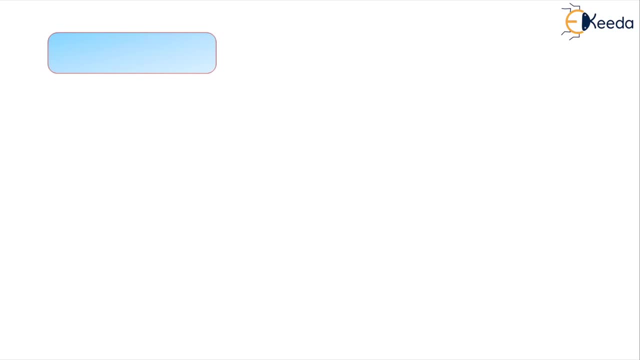 Those are required. First of all, let us discuss, with respect to The coding redundancy here, The first type. So let us assume that Each sample of the discrete time signal in general, If it is represented as x of n, Will be a random variable. r suffix i. 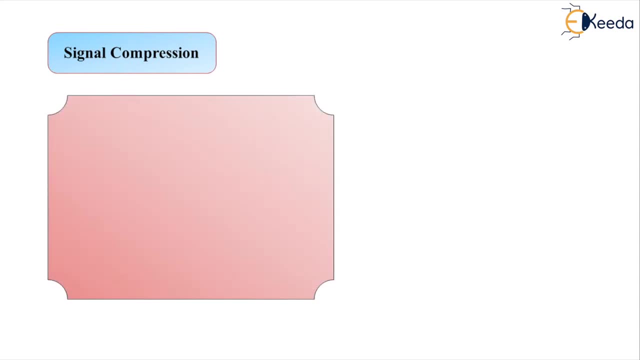 Taking one of capital q- distinct values, With the probability denoted by p suffix i. So this i is greater than or equal to 0. But less than or equal to capital q minus 1. here. Now here the representation of p suffix i. 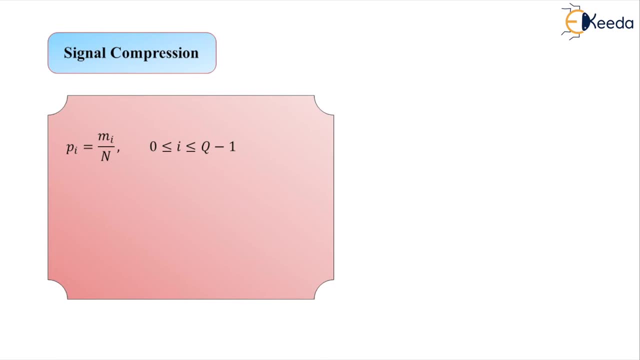 Will be less than or equal to 1.. As this is the probability, It will always be less than that of the 100% I can say, And the summation for i is equal to 0 to capital q minus 1.. 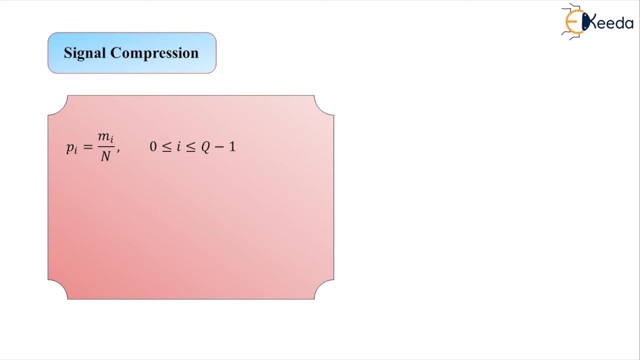 Of this probability, As discussed, will be equal to 100%, That it is 1 here. So each possible value R suffix i is usually called as A symbol in general, And the probability p suffix i Of each symbol r suffix i. 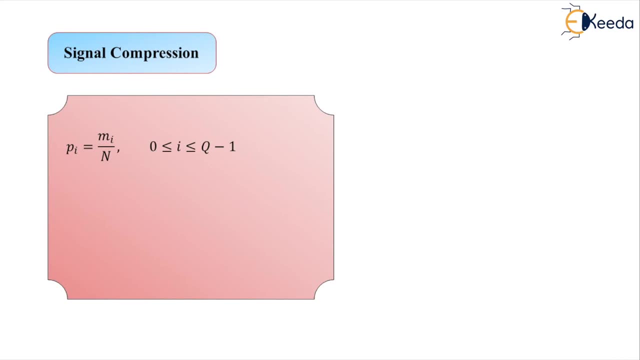 Can be estimated from The histogram of the signal. Histogram is plot of the information For how many number of times A certain value comes to The signal information Versus the Different gray levels If it is a concern of image. 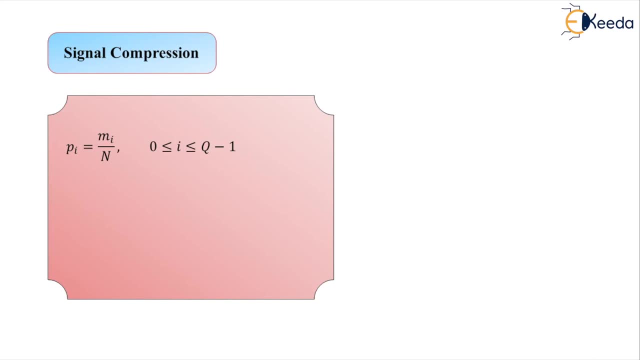 Or the signal representation With the help of particular bits here For coding purpose here. So therefore, If the signal will contain A total of capital q minus 1.. A total of capital n- number of samples, With m suffix, i Denoting the total number of sample. 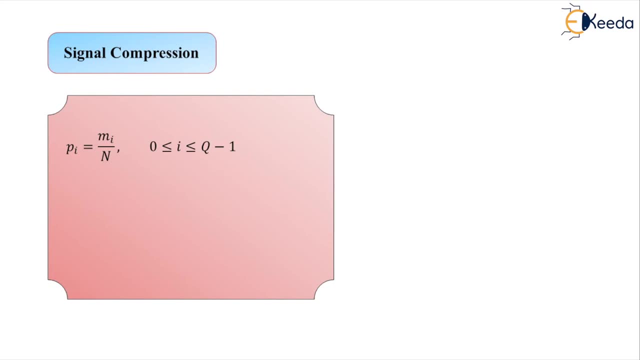 Taking the value of R suffix i, We have this representation: P suffix i is equal to m suffix i Divided by capital n here. So let us have The representation b suffix i To be the length of The ith code word. 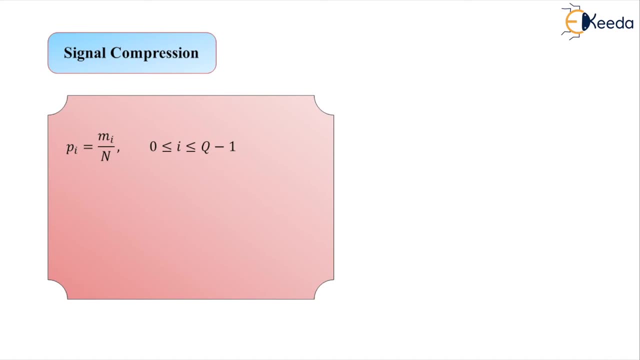 That is the total number of bits Necessary to represent the value Of the random variable r. suffix i, So that time A measure of coding redundancy Can be given by The average number of bits Needed to represent each sample Of the signal x of n. 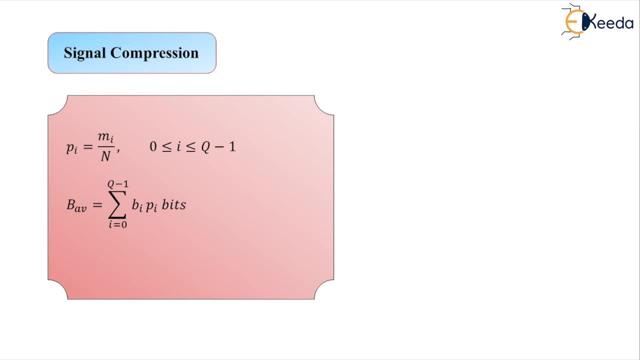 So here we denote Capital b suffix av, Av. for the average That is equal to the summation I is equal to 0 to capital q minus 1.. Or the product of b suffix i With p suffix i In terms of bits here. 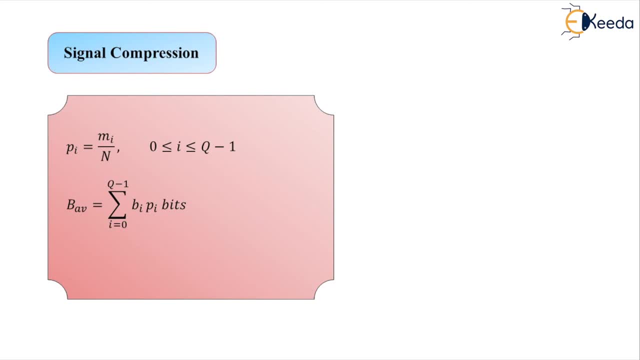 The total number of bits Required to represent a signal Can be capital n. Multiplied to this representation, Capital b suffix av. here Now, along with This important two formulae, Let us discuss with respect to the Entropy, as it is very, very. 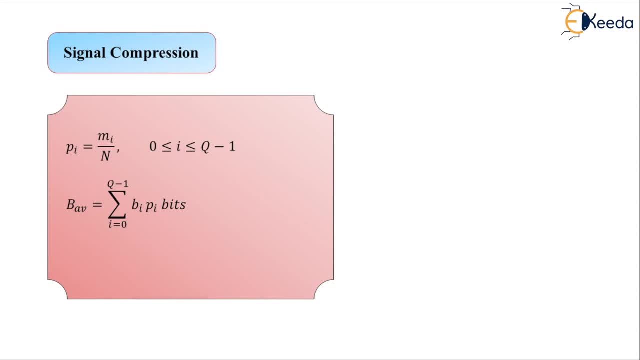 Essential parameter Associated to the signal compression Here see. The goal or the objective Of signal compression methodology Is for reducing The volume of the data, While at the same time There should be preserving The information quality Next to the original signal. 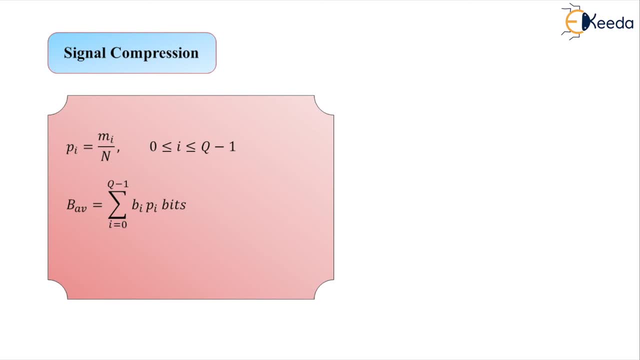 With some acceptable Fidelity also. So the information content Represented by a symbol Can be informally related To its unexpectedness. That is, if a symbol Arrives is one That we call expected, And if Unexpected symbol will arrive. 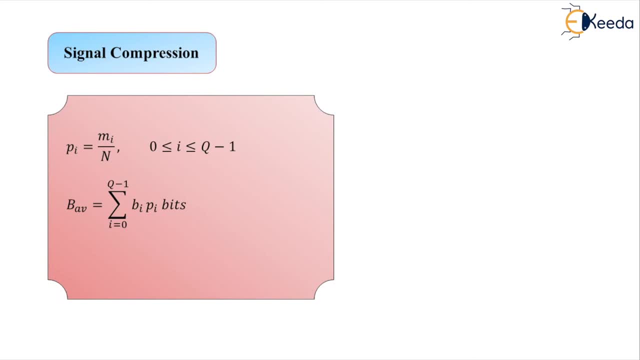 It will convey Much more information That it was not the case of the earlier. So therefore, the information content Of a particular symbol Can be related to its corresponding Probability of occurrence. So for the discrete time, sequence X of n with samples. 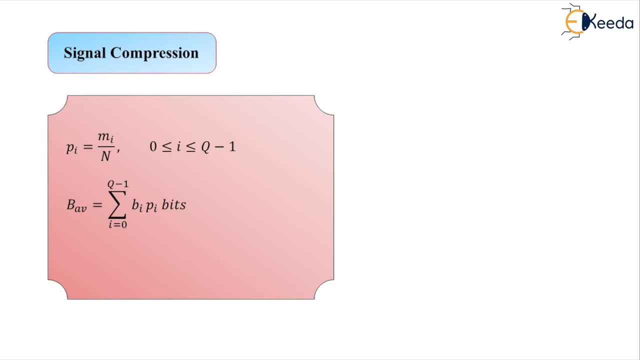 Taking one of capital Q, distinct symbols ri, With the probability pi as shown, The first equation: here We have a measure of The information content Denoted by capital I. suffix small i That is given as Minus log to the base 2.. 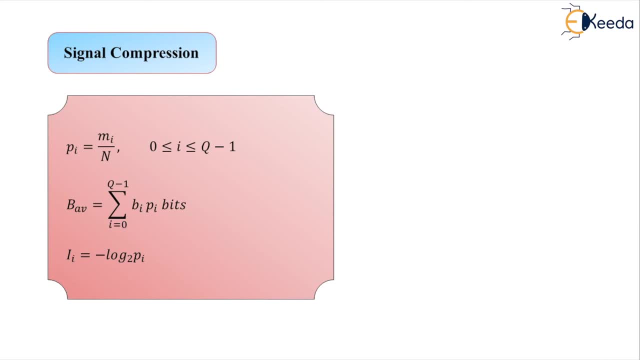 Of the probability p suffix i. So from this representation It follows that the information Content capital I suffix i is always Greater than or equal to 0. And also It can be seen that The information content I suffix i is very large. 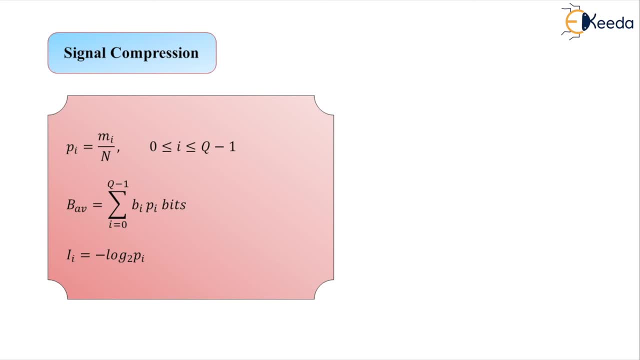 So in short, That it is the inverse Relation between the probability And the information content. here Now a measure of The average information content Of the signal x of n Can be given by corresponding entropy, Which we have denoted by. 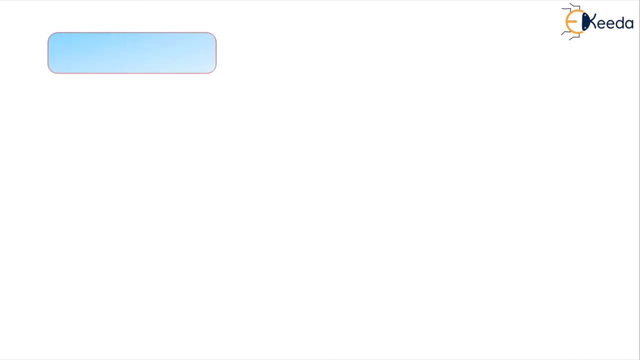 Capital H suffix x. X is the signal here, So hx is equal To the summation, I is equal to 0, to capital Q minus 1, or Probability p suffix i With the information content: I suffix i. So this is expressed as: 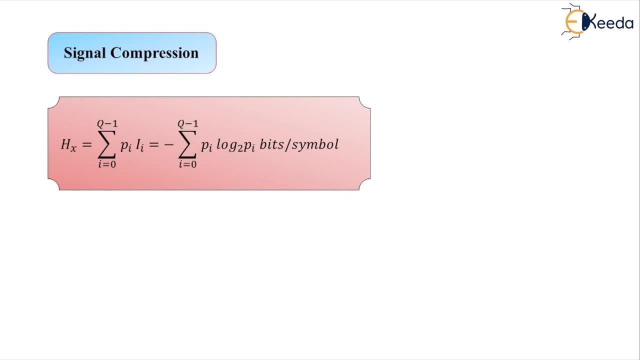 Minus the summation Or index variable, I is equal to 0. to capital Q minus 1 or p suffix i Multiplied to log to the base 2.. Of p suffix i In terms of bits per symbol. So this is the coding redundancy. 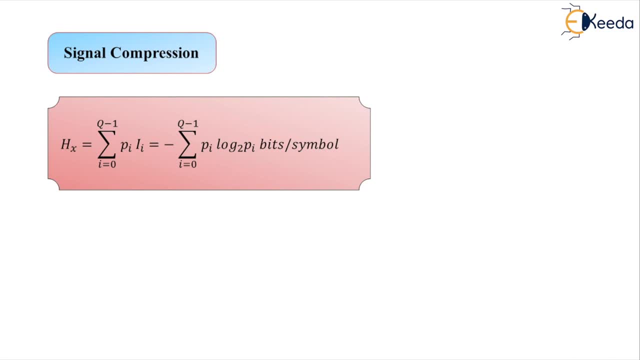 As we discussed The difference between the actual data rate And the entropy of The stream here. So this was our topic: The signal compression. So this was our 8th video From the 8th chapter That it was applications of signal processing. 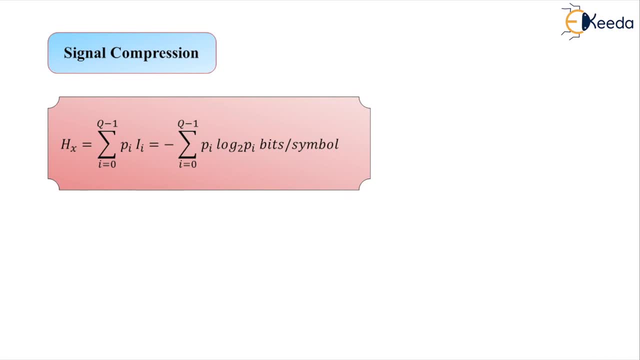 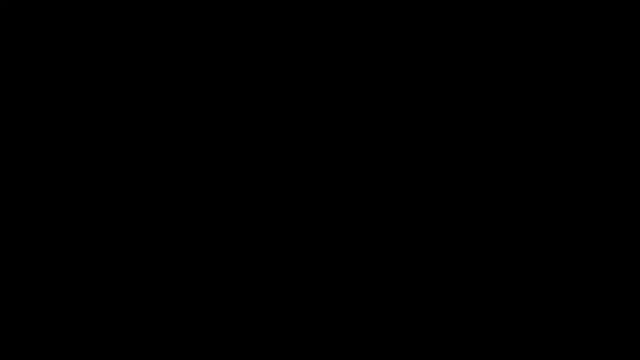 By the next lecture We shall have continuation into the same To discuss one more application, That is of trans multiplexers. Thank you, Thank you.